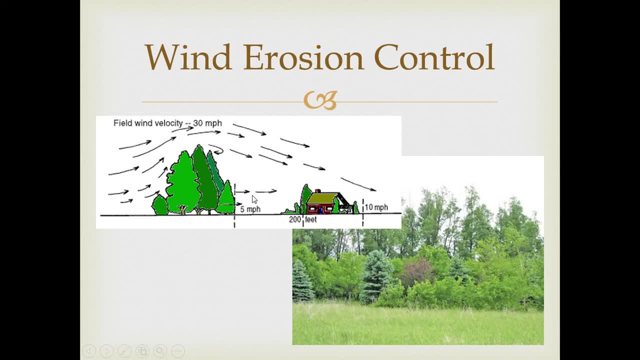 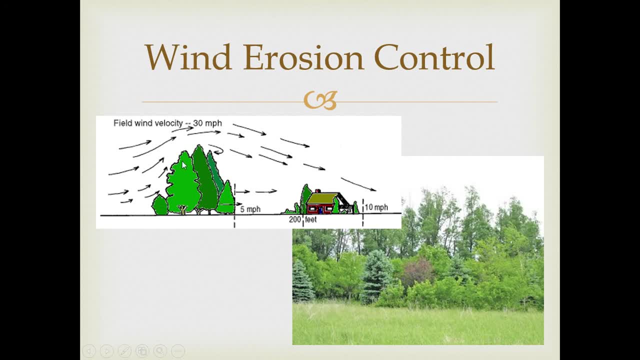 10 mile per hour. so if you're installing a wind break, it's important to sort of plan your distance, whether it's a structure or a field or a road, you know, we want to make sure those are placed appropriately. and then down here just have a picture of a multi-species sort of multi-generation. 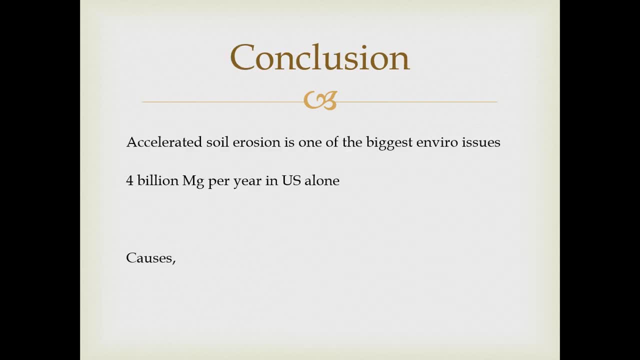 windbreak so that it'll always be present on site. so erosion conclusion: accelerated soil erosion is one of our biggest environmental issues. over four billion megagrams of soil per year in the us alone. that's about check our units here. hundreds thousands, millions, billions, trillions. 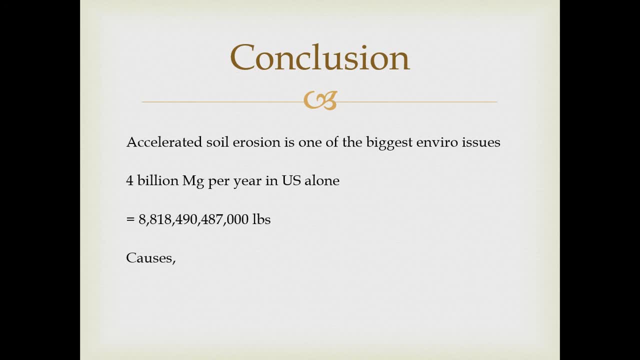 8.8 trillion pounds of soil is eroded in the us annually, causing by wind, water and tillage. so those are kind of our three soil erosion factors and things that we need to manage. so most effective controls, again, limiting exposure, no bare soil, protecting it with whether. 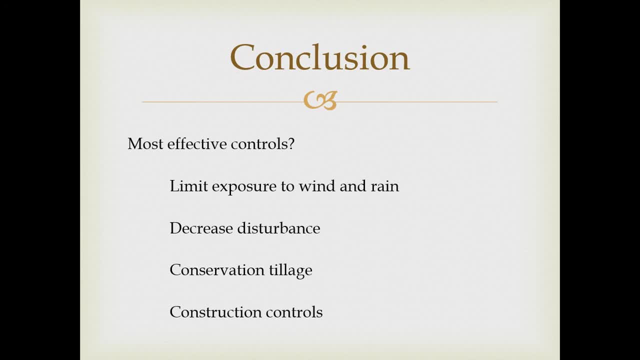 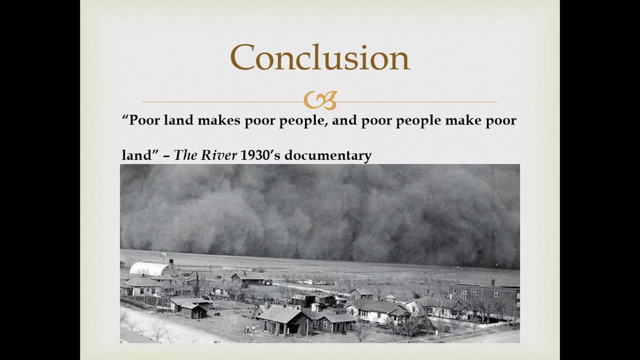 it's plant material or just some other physical barrier from wind and rain, decreasing disturbance, just in general. again, keeping soils covered. you can do that through conservation, tillage and through construction controls, and we have examples of each in previous videos and science to support their use. and conclude with a quote from the river which was about the dust bowl. 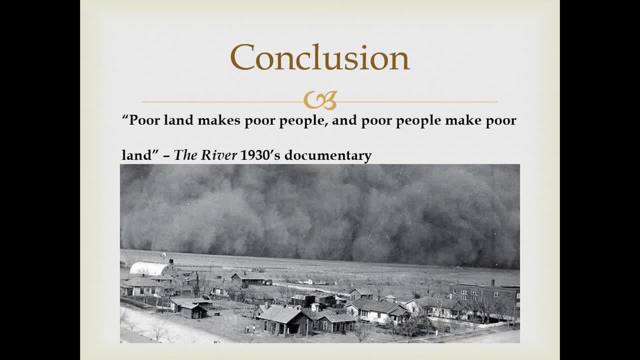 1930s, poor land makes poor people and poor people make poor land, and so hopefully a theme you picked up in these erosion videos was this: um sort of feedback loop of degradation causes erosion which causes more degradation, and how we just sometimes need to step up and front the cost of protecting soils and that feedback loop. 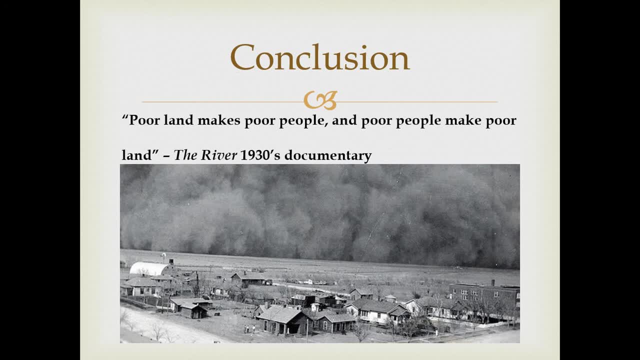 then comes into our favor. so if we can protect the soil, the soil gets healthier, our plants get healthier and we're able to protect the soil better.